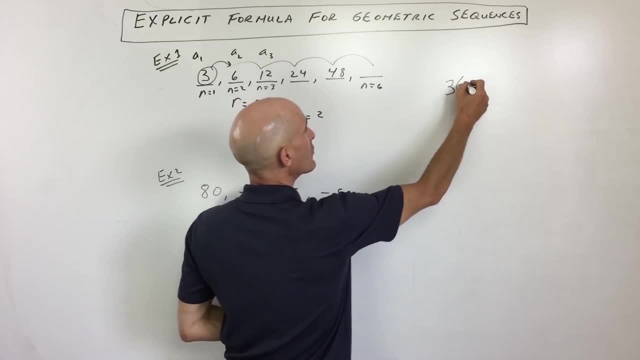 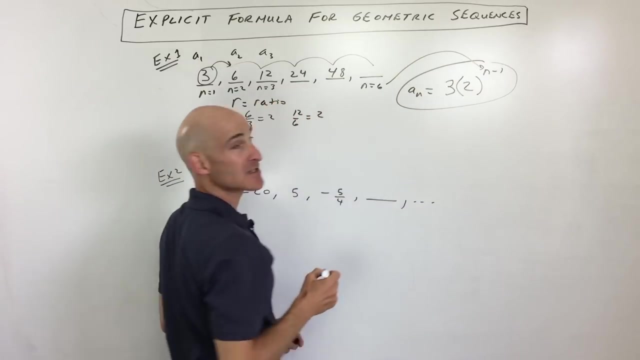 about what we just did. we took the first value, which is three. we multiply by two n minus one times. okay, So in this case, that's our formula. So a sub n equals three times two to the n minus one. Now, if we wanted to find the sixth term, what we would do is we would put six in place of 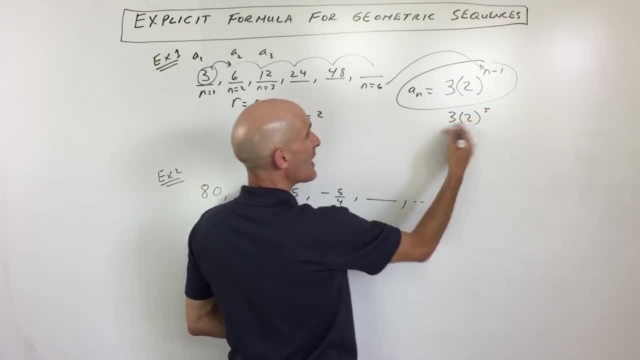 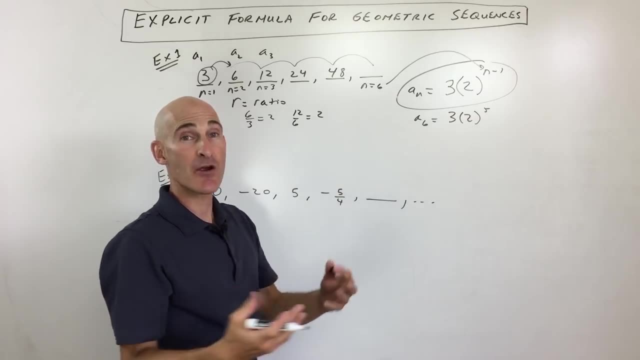 n. So this would be three times two to the fifth, and we can simplify that, and that's going to be the value of our sixth term. okay, Now to write this in a more, you know, generic way, so that you: 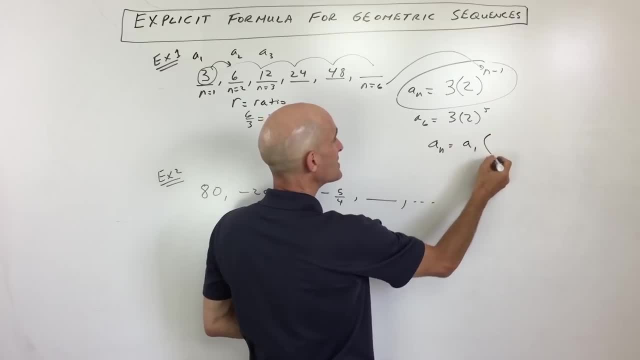 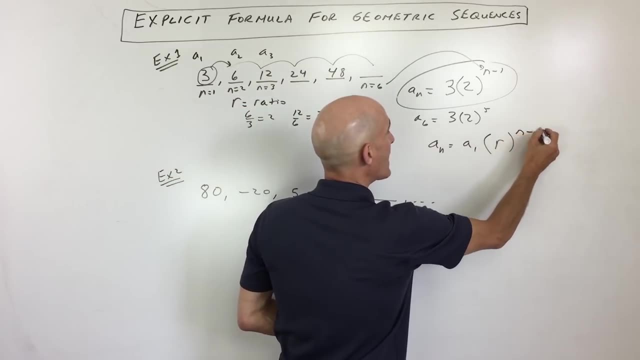 can use it. here's your formula, right here It's: a sub n equals a sub one. that's the value of the first term times r. that's your common ratio. that's what you're multiplying by to get to the next term, to the n minus one power. It's always one less, okay, So that's your formula. So 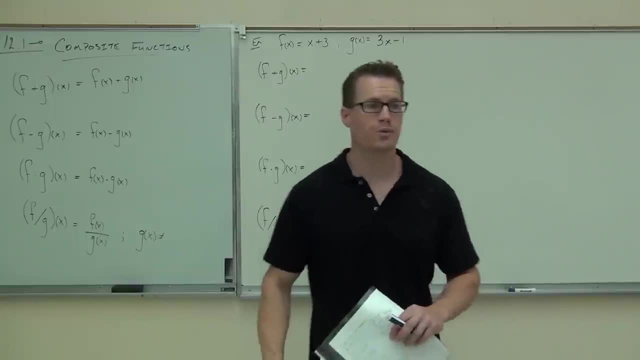 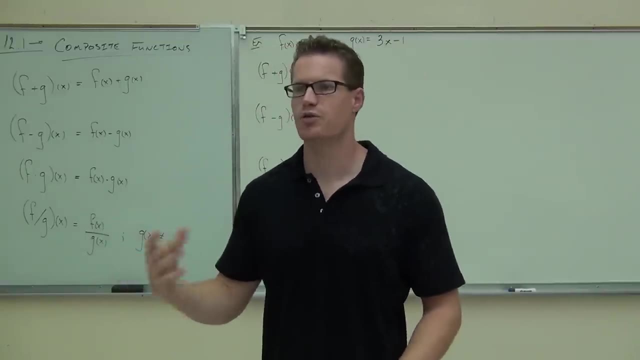 So in chapter 12, we're all about functions, and in 12.1 and 12.2, we introduce a few concepts about functions. Now we've been dealing with functions for a long time. Functions are just these things that we can graph on an x-y axis. Typically, our functions were linear lines. 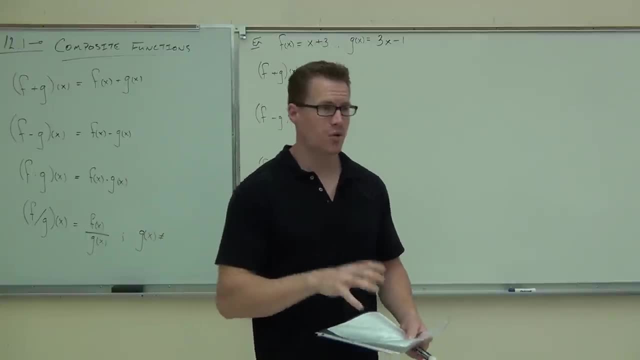 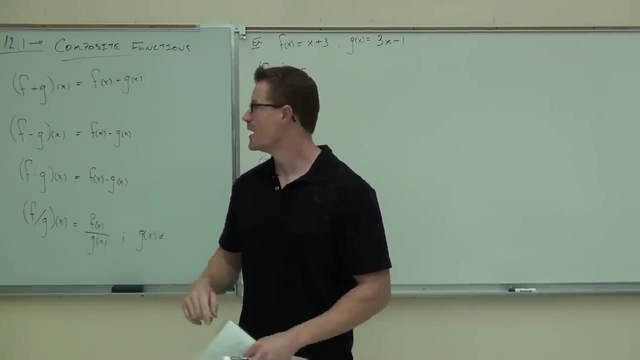 or quadratic parabolas, and we just finished a whole chapter about graphing and working with quadratic functions. That was what your homework was on from last time was graphing those parabolas. yes, Cool, all right. Well, now we can learn a couple things about functions. 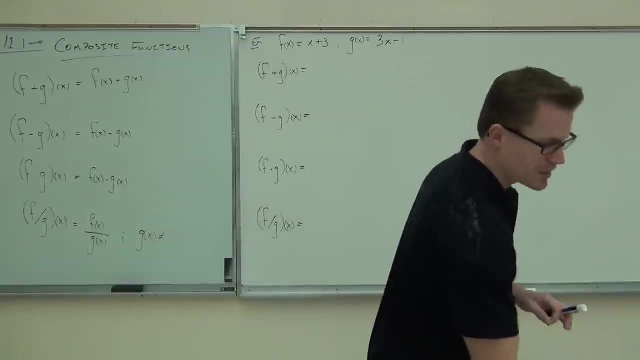 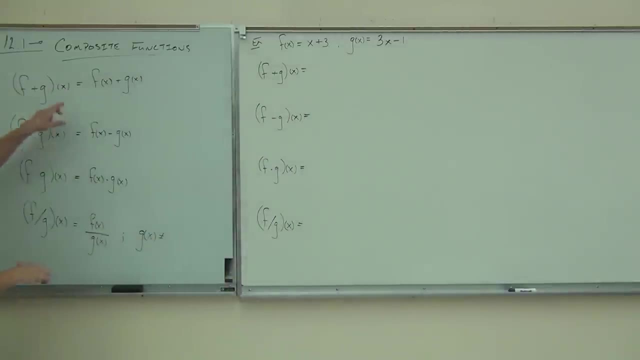 in general. The first thing that we need to know about functions is that we can add, subtract, multiply and even divide two functions. Here's what all this means. I've already put this on the board for you, but this just says if I want to add two functions. by the way,